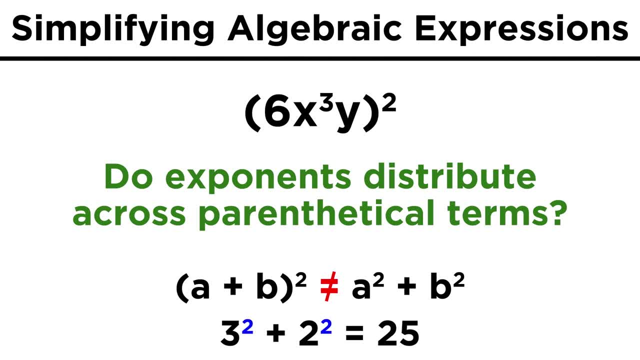 try to distribute the exponent. three squared plus two squared is nine plus four or thirteen, so we clearly weren't allowed to do what we did. To evaluate the square of a sum we need another technique that we will learn later, but a 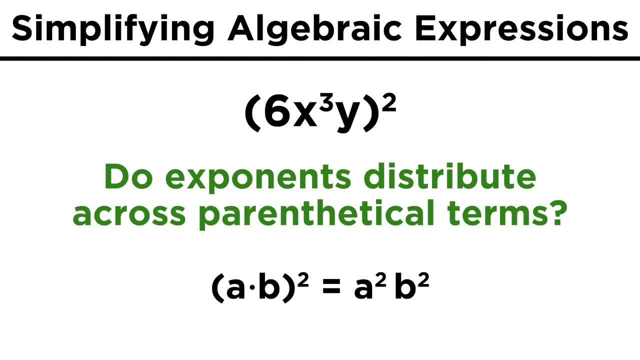 times b. quantity squared is indeed equal to a squared times b squared. This is easy to prove because a- b squared is a b times a b and since multiplication is associative, we can shuffle these around to get a, a, b b or a squared, b squared. 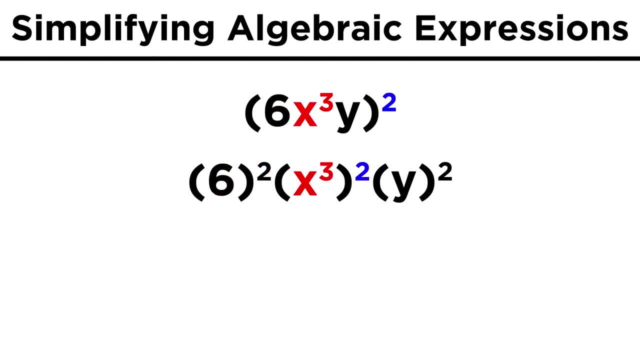 So we can look at this term and rewrite it as six squared times x cubed squared times y squared. Now we continue to simplify. Six squared is six times six, or thirty-six For x cubed squared. let's remember that x to the a to the b is equal to x to the a. 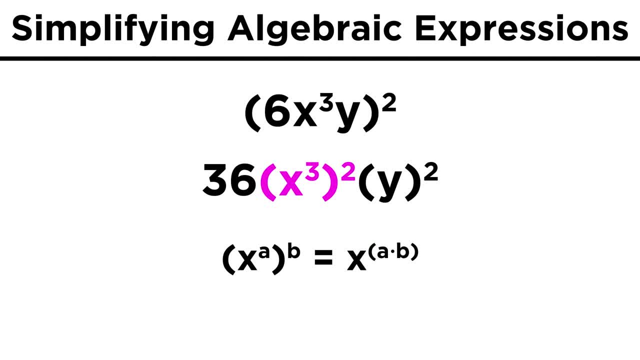 times b, meaning that we multiply the two exponents together. That means x to the three times two, which equals six, or x to the sixth, And y squared stays as it is. So we are left with thirty-six x to the sixth, y squared. 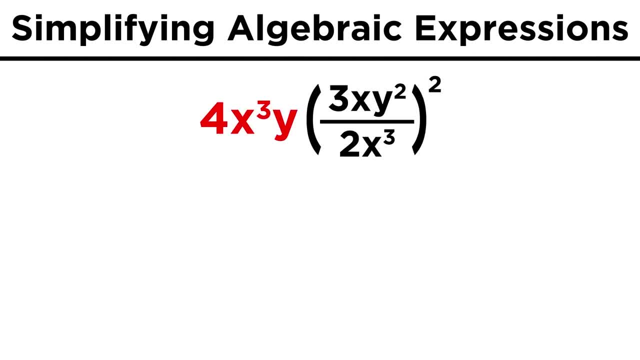 Let's try a trickier one. We have four x cubed, y times this fraction. in parentheses, Three x y squared over two x cubed, all of which is squared. The first thing we want to do is distribute this exponent over everything in the fraction. 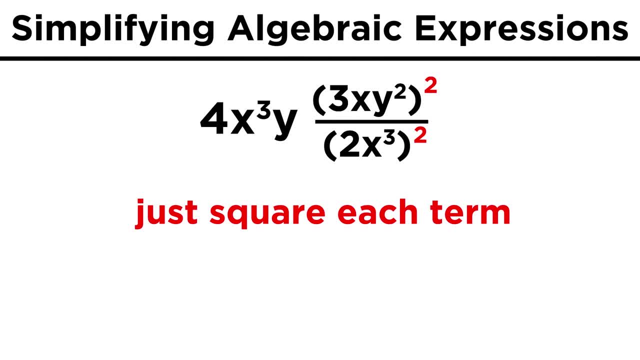 If the whole term is squared, then each individual term can be squared: Three x y squared becomes nine, x squared, y to the fourth. and two x cubed becomes four, x to the sixth. Now we can combine like terms for this term on the left and the numerator of this fraction. 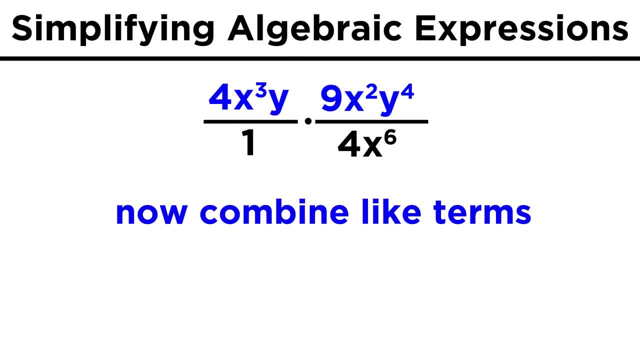 Remember that when multiplying a fraction by a number, the number only multiplies the numerator, and this is no different. Four times nine is thirty-six. x cubed times x squared is x to the fifth and y times y to the fourth is y to the fifth. 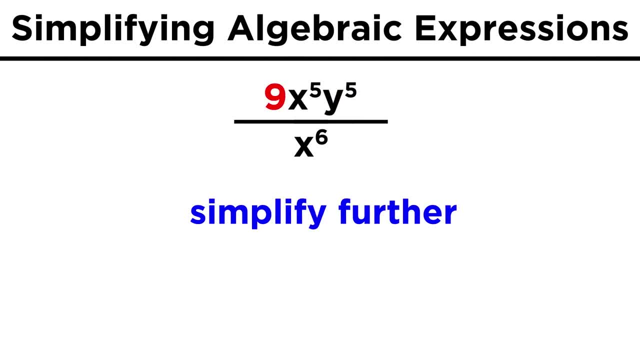 Now we can simplify a bit further, since thirty-six divided by four is nine, and x to the fifth divided by x to the sixth is x to the negative one, since five minus six is negative one, This is the same as leaving x in the denominator, because x to the negative one is the same. 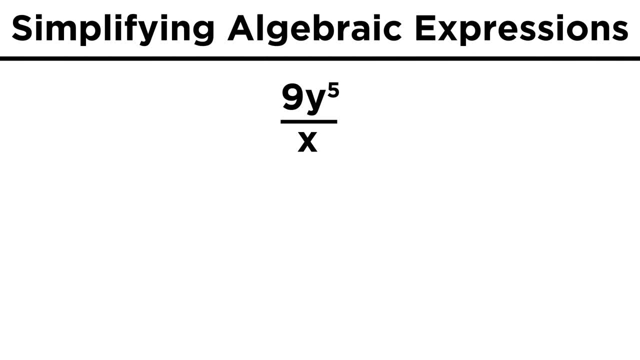 as one over x. So we are left with nine y to the fifth over x. How about this? one x to the sixth over sixty-four, all raised to the negative two-thirds power. There are a few ways to approach this, but let's first address the fact that the exponent 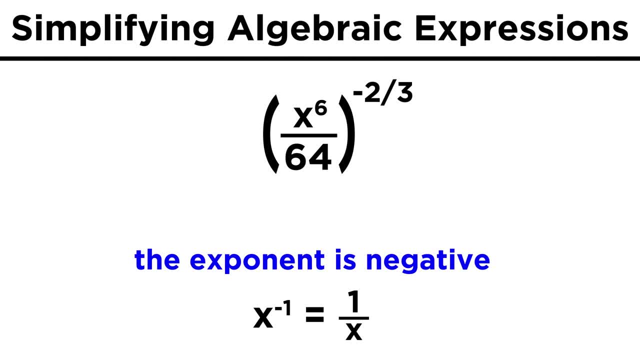 is negative. If this were a single term, we could put one over the term and then make the exponent the exponent positive, the way we said that x to the negative one is one over x. But since we already have a fraction, let's just flip it over. 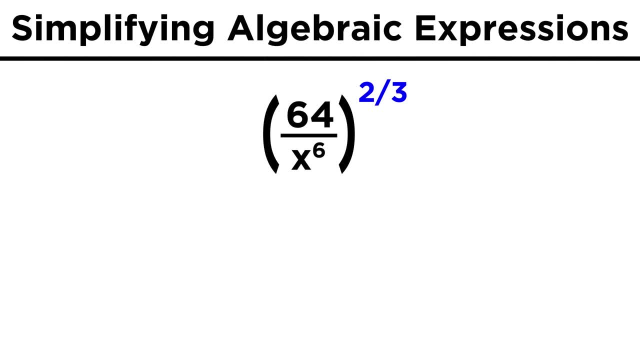 If we turn this upside down, we can change the exponent to positive two-thirds. Now, as we recall, raising something to the two-thirds power is the same as squaring it and taking the cube root in some order. Since it's easier to work with small numbers, let's take the cube root first, making sure. 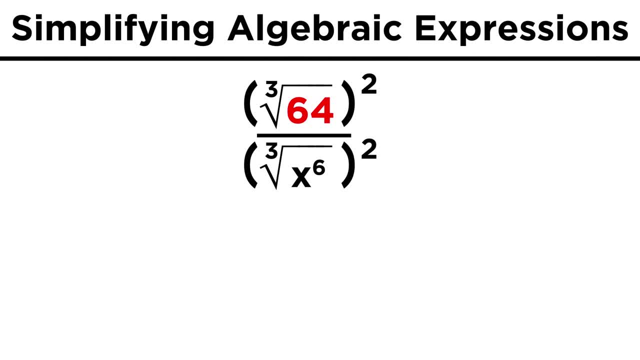 to do it for both top and bottom. The cube root of sixty-four is four. The cube root of x to the sixth, which is like x to the sixth to the one-third, is equal to x to the sixth times one-third, which is two. 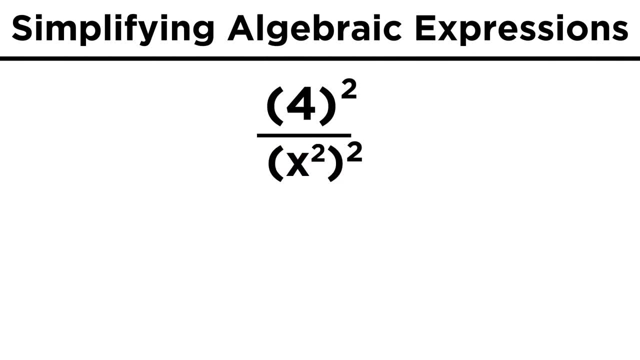 So we get x squared. That takes care of the denominator of the exponent. so now we just square the top and bottom. That leaves us with sixteen over x to the fourth, which can't be simplified further. Let's try another Ten a to the two x plus y. 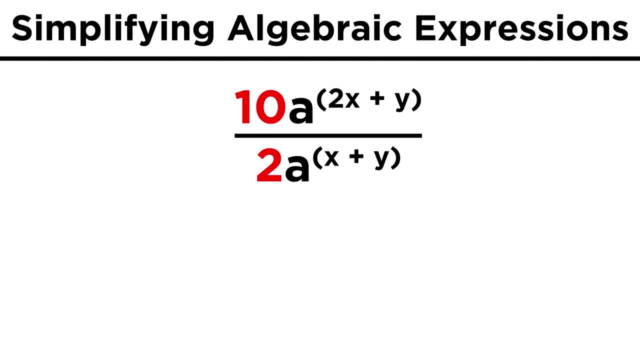 Here we can see that ten over two can be done separately, which gives us five. Now to deal with this part of it again, we can just use the rule for dividing some base raised to two different exponents. We just subtract them. So a to the two x plus y over a to the x plus y gives us a to the two x plus y minus the. 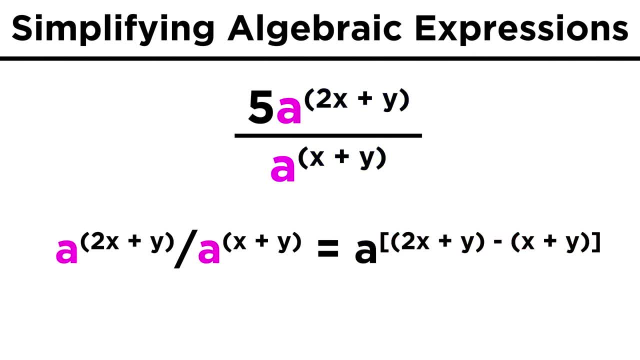 quantity x plus y. This only works because a is the base in both terms. If the bases were different, we couldn't do this. Then remember that we have to subtract the entire exponent in the denominator, so we need parentheses to do this.